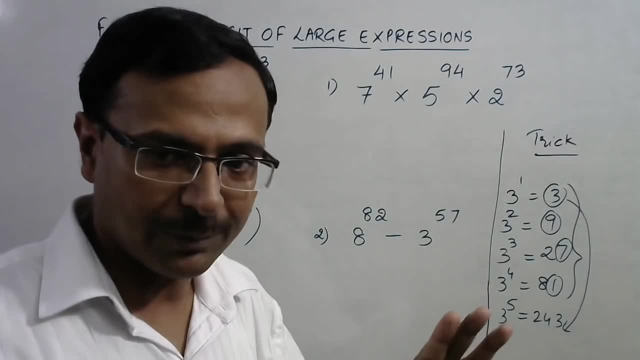 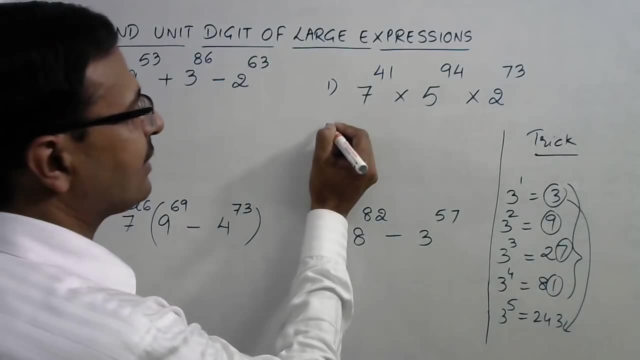 If you are left with, If you are left with 2, then unit digit will be 9, and so on. So this is the trick I am going to use and it is applicable for all bases. Like here: we have 7 raised to power 41, so this is actually 7 raised to power 4 into 10, this is 40.. 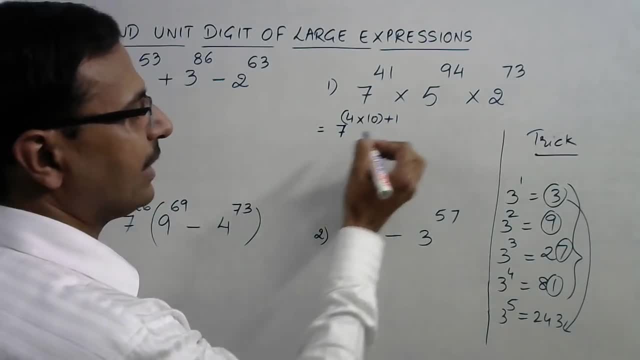 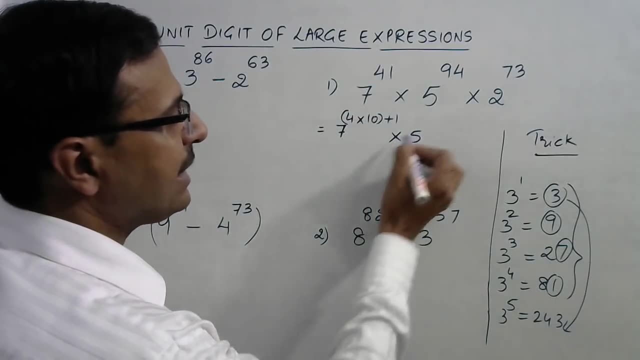 So this will get eliminated and you have only plus 1.. So this is 41, so we will eliminate this and this will be 7 raised to power 1, only Then 5 raised to power 94,. 94 means 4 into. 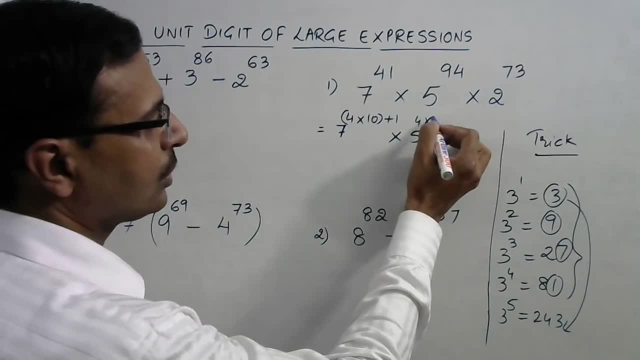 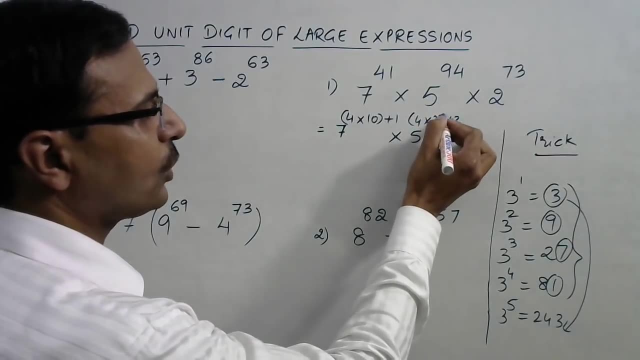 Now this is 24, okay, 24 into 4 is 96,. so 23 into 4,, 92 and plus 2.. So this 4 into 23,. we will eliminate from here and we will have only 5 raised to power, 2 left behind. 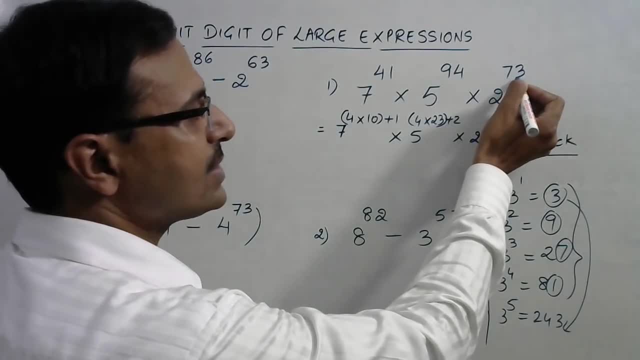 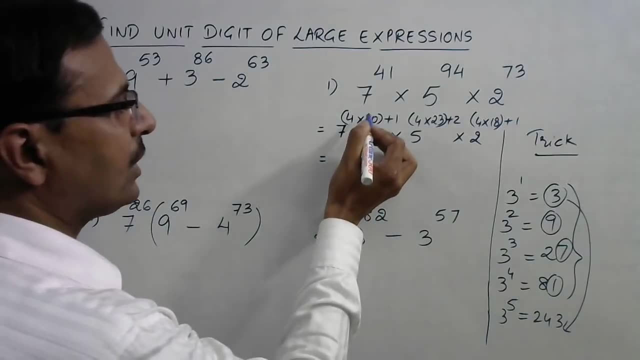 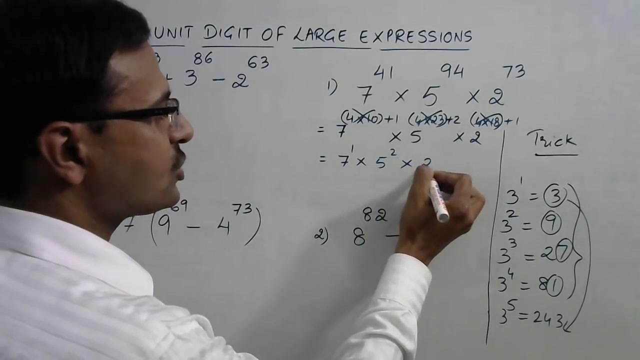 Similarly, we have 2 raised to power 73, we know that 72 is divisible, So 4 into 18 is 72 and we have one more power. So now eliminate all these multiples of 4s. So we have 7 raised to power 1, 5 raised to power 2 and 2 raised to power 1.. 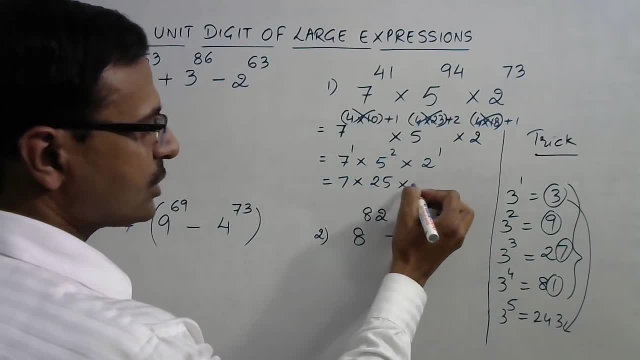 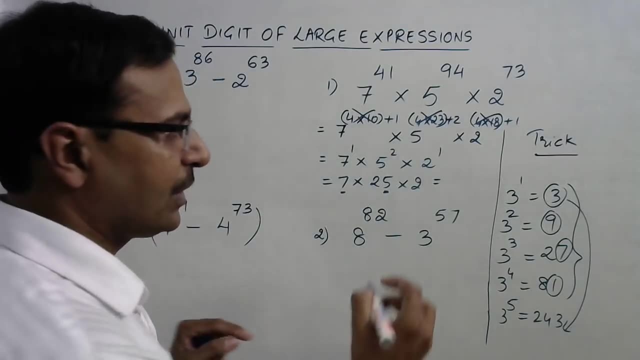 Now, 7 into 5, square is 25, and 2 raised to power 1 is 2.. Now you can find the unit digit very easily: 7 into 5, 35, so we have unit digit 5.. Now 5 into 2, 10, so unit digit will be 0.. 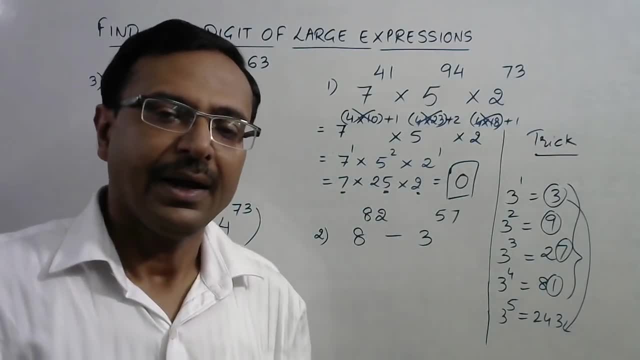 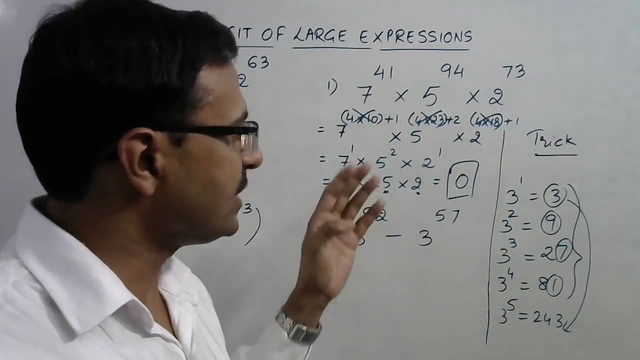 So your answer for the question is 0.. If you do not follow this method, then 5 and 2, if they occur together, then you will. Unit digit has to be 0 only, But in this case you have proved that the unit digit is 0. 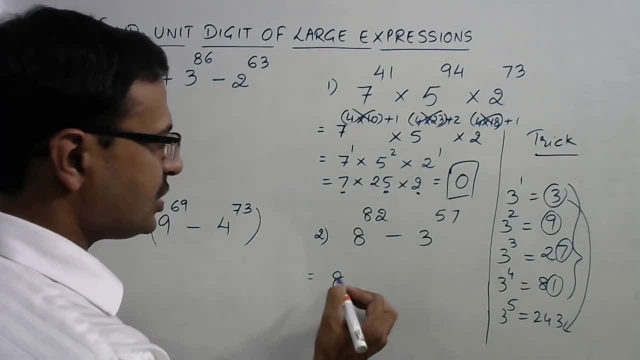 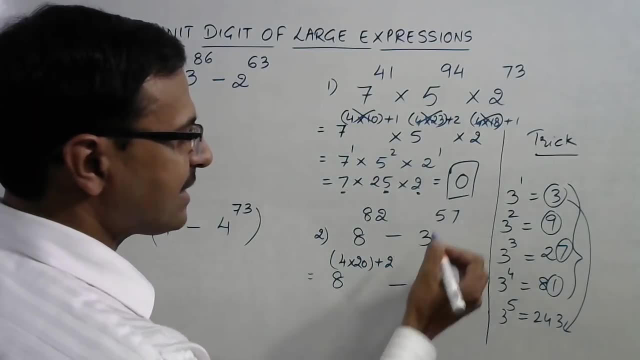 Let's see this question Now. see 8 raised to power 82.. 82, 4 into 20 is 80 and you are left with plus 2, this is 82. And 3 raised to power 57,. we all know that 56 is divisible by 4.. 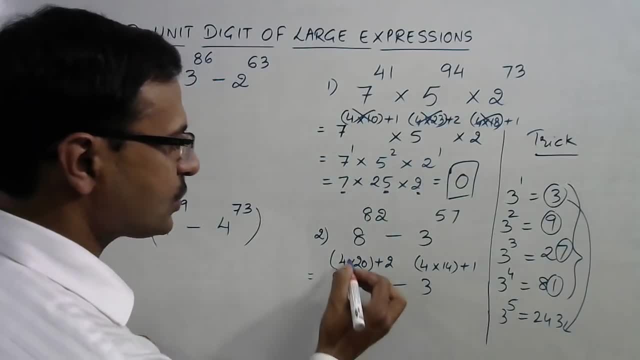 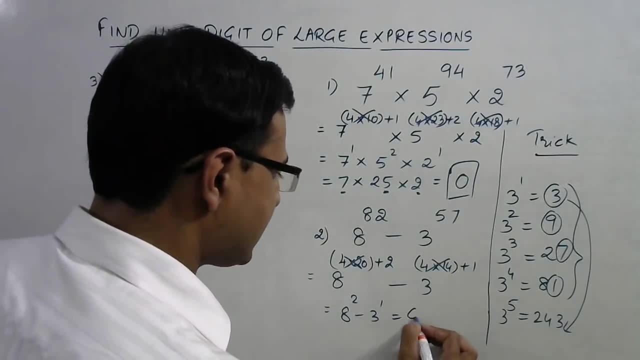 So 14 into 4 is 56 plus 1, 57.. So eliminate these multiples of 4.. You have 8 raised to power 2 minus 3 raised to power 1.. Now 8 raised to power 2 is 64.. 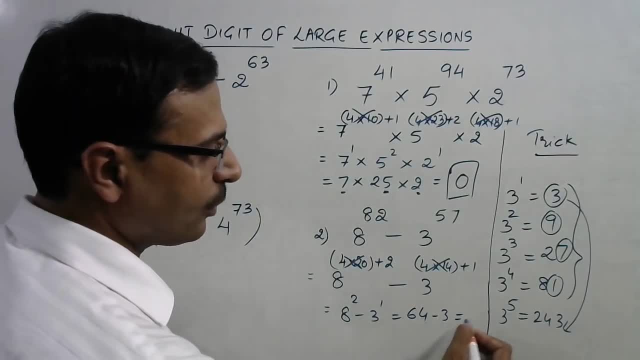 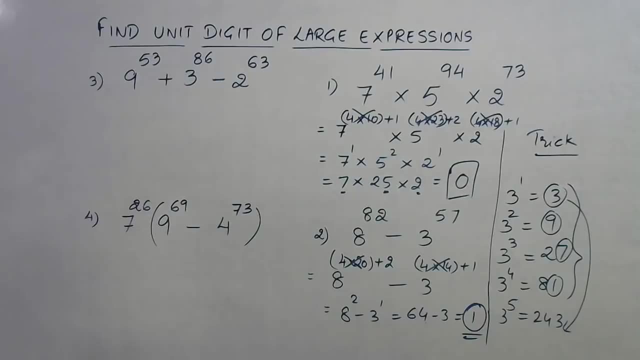 So you have 4 here and 3 here. So unit digit will be 4 minus 3, 1.. So in this case you will have unit digit 1.. Likewise you can find the unit digit here: See 9 raised to power something. so 9 raised to power 53.. 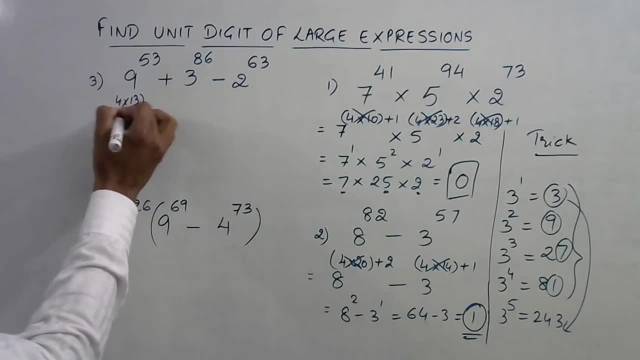 So 52, 4 into 13 is 52 and you have 1 left out. Then 3 raised to power 86,. 4 into 21 is 84 plus 2, 86.. And 60 is divisible, so 4 into 15 is 60 plus 3.. 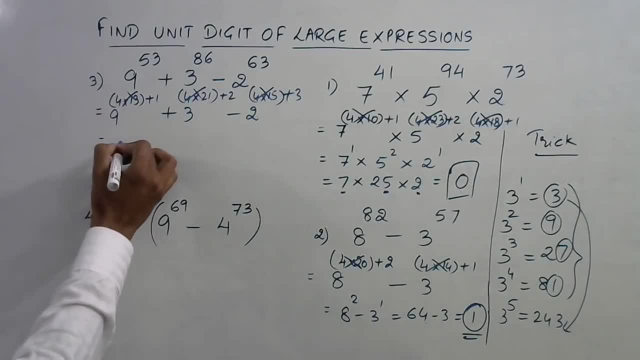 So now I am eliminating all multiples of 4.. So this is 9 raised to power 1,, 3 raised to power 2, 2 raised to power 3.. So this is 9 plus 9 minus 8.. 9 plus 9 is 18,, 18 minus 8.. 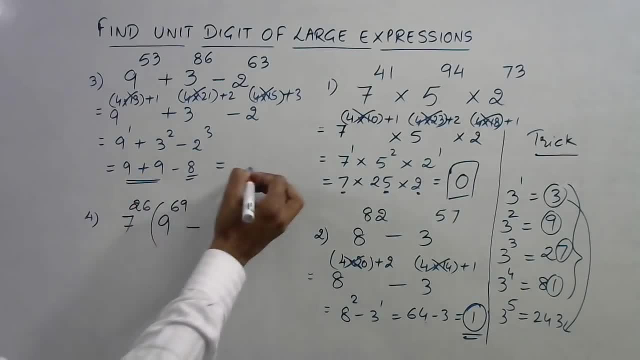 You have 9 plus 9 is 18,, so unit digit is 8.. So 8 minus 8 is 0. So unit digit will be 0 in this case. Likewise here, 7 raised to power 26,, 24 is divisible by 4.. 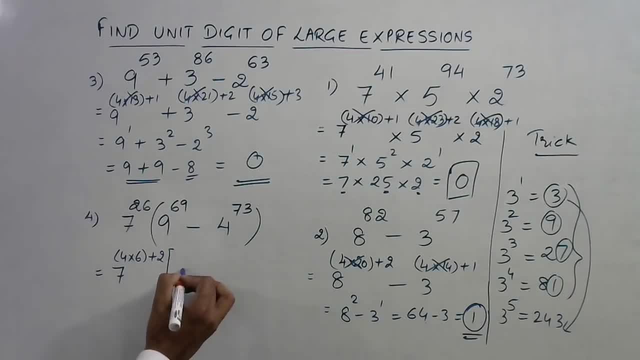 So 4 into 6 is 24 and you have 2 left out, Then 9 raised to power 69.. 69 means 17 into 4 is 68 and 1 left out. Here we have 4 into 18, 72 plus 1 left out. 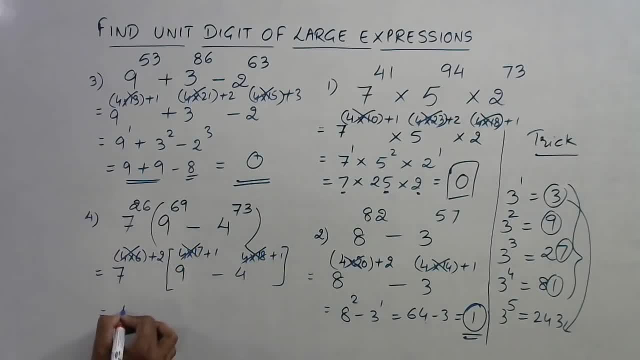 So eliminate all powers, all multiples of 4.. You have 7 square 49 and this is 9 minus 4.. So this is unit digit is 9 here And 9 minus 5,. 9 minus 4, 5 here. 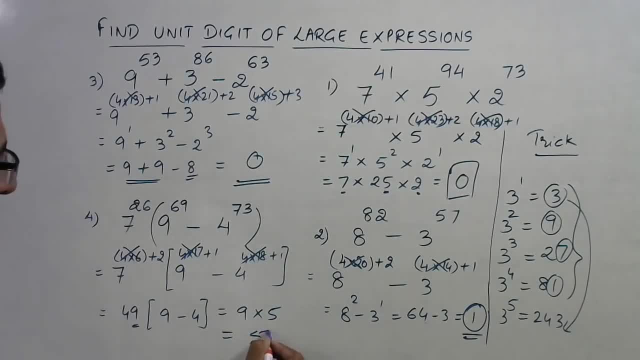 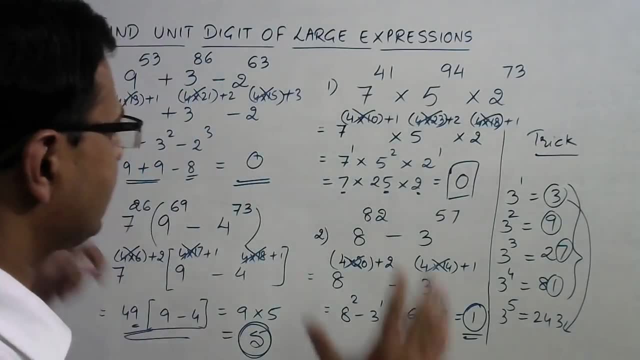 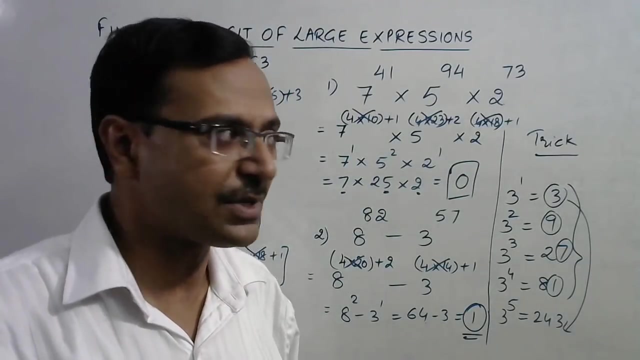 So 9 into 5, 45,, thereby giving you a unit digit of 5.. So this is not an actual calculation. We just want to find the unit digit in order to find the unit digit of the large expressions like this. So, friends, this is the way you need to find the unit digit of large expressions. 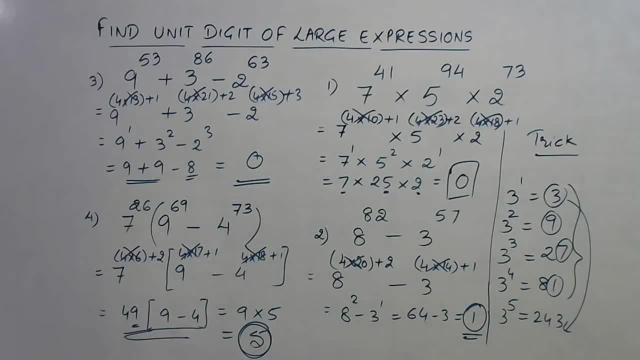 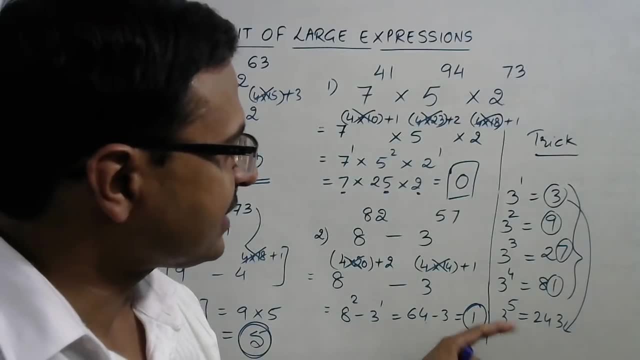 And you should have this knowledge of this useful trick that the power you know, when you take 4 powers, then in the 5th power the unit digit will take 4.. It repeats itself In the 6th power. you will have same power, same unit digit as power 2, and so on. 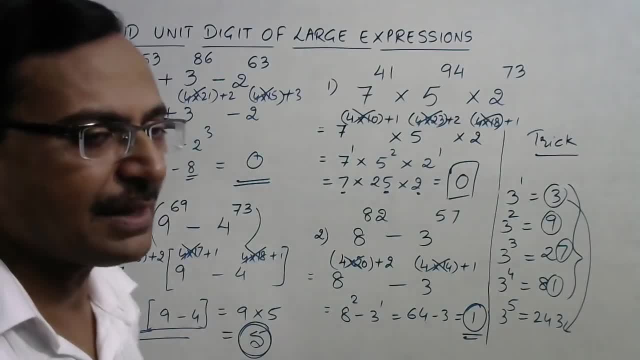 So, friends, you like this video, Very useful for competitive exams. Do share it with all your friends And do not forget to subscribe the channel for more uploads.